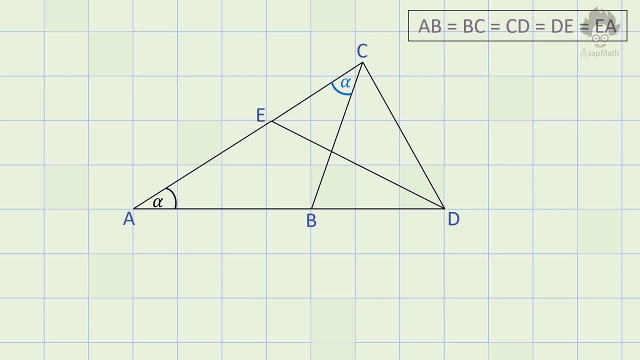 of a triangle is equal to the sum of the opposite interior angles. So here, angle CBD equal sum of angle B, A, C and A C, B. Therefore we know angle CBD equal to alpha. Moving on to second criteria: BC equal CD. Now again triangle: BCD is an isosceles triangle. 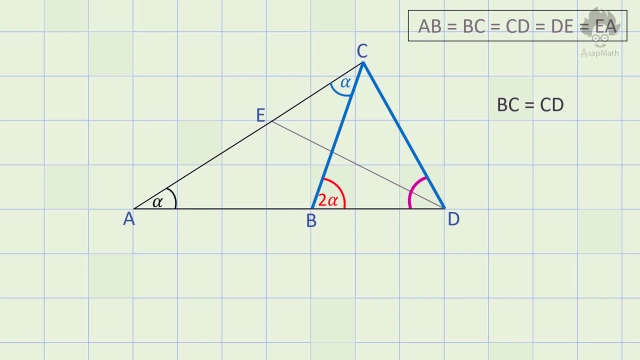 As opposite angles are equal, angle B, D, C is equal to 2 alpha. Now we know two angles in triangle BCD. Therefore angle is sigma量 in angle BCD. Hence we can find the angle BCD. Sum of interior angle of a triangle is equal to phi. 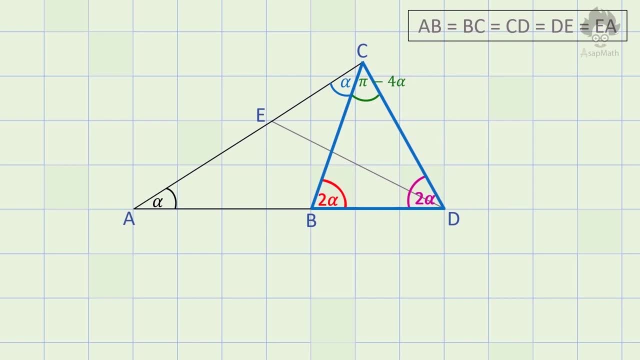 So angle BCD is equal to phi minus 4 alpha, As angle ACB is alpha And angle BCD is phi minus 4 alpha, And angle BCD is phi minus 4 alpha And angle BCD is phi minus 4 alpha. 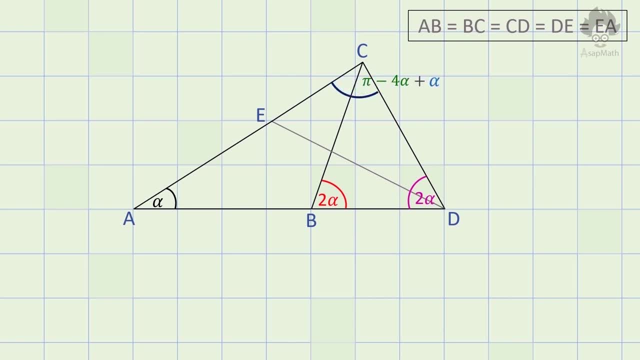 combining these two can get angle ECD. Angle ECD is equal to phi minus 3 alpha. Now if we consider the third criteria, CD, equal DE- it again shows that triangle CDE is an isosceles triangle. So angle CED is equal to phi minus 3 alpha. 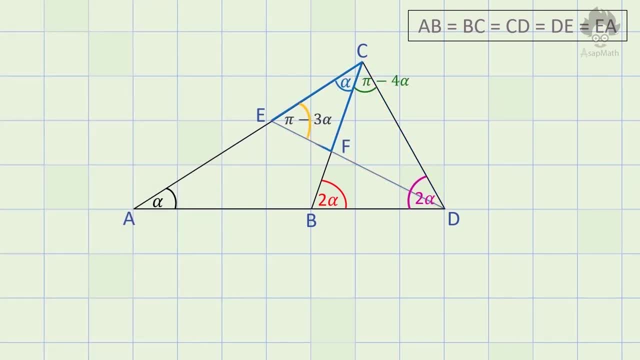 In triangle CFE also, we can find the remaining angles, as we already know, two angles. So angle CFE is equal to 2 alpha. As angle CFE and BFD are opposite angles, they are equal, So BFD is equal to alpha.